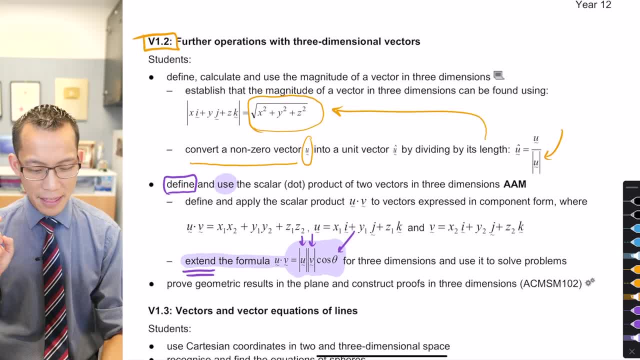 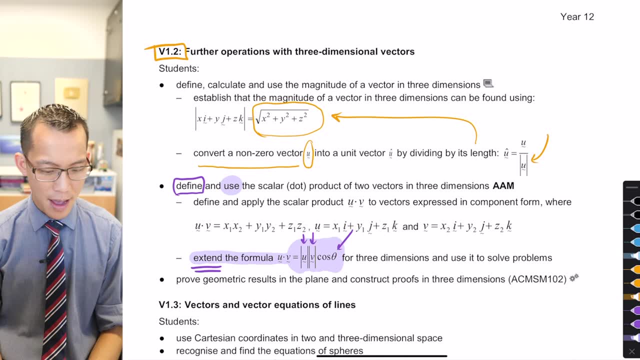 vector equations of lines next week. Now, the thing that we're going to do today is a little bit like remember I told you about ratio division, Ratio division doesn't explicitly come up anywhere here, but it's a really great way to learn some of the skills that the syllabus 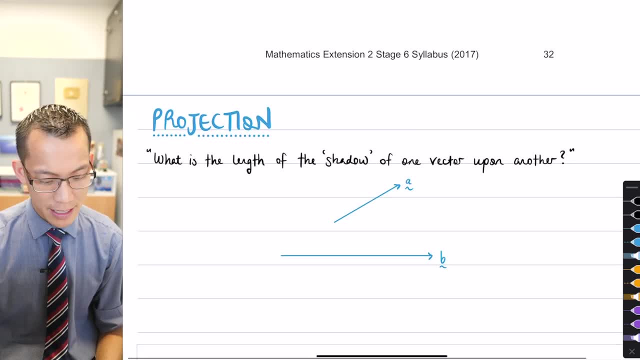 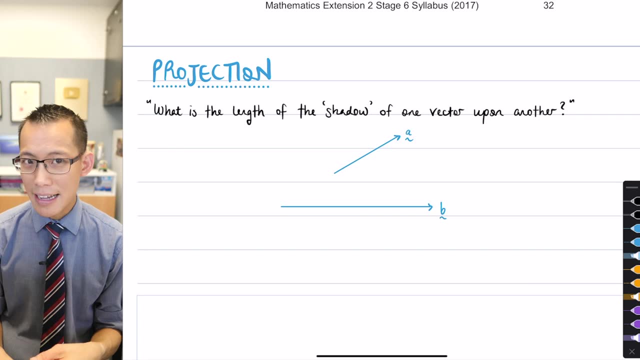 wants of us, right. So I'm going to be doing much the same thing today with this idea of projection. It's not explicitly mentioned, it's just such an applicable idea. It's very clever. It builds on what we've done in extension one. I know you've met projection before, but what I'm going to do is I'm kind of 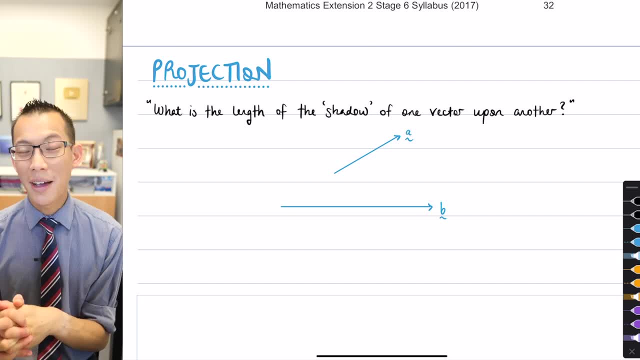 going to expect. maybe this is an unfair expectation, but I'm kind of going to expect that you know maybe the formula for projection. Don't worry, I'm not going to ask you to recite it. There are multiple ones if you remember that, but perhaps don't have much of the understanding. 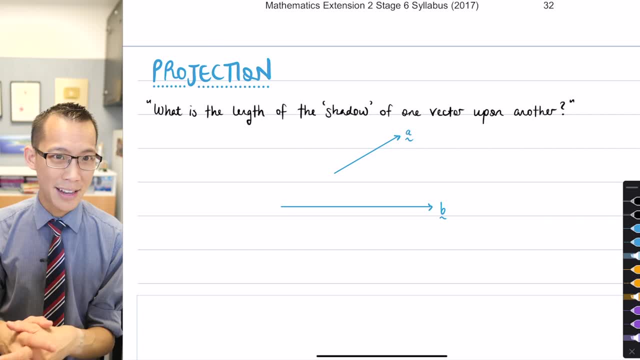 about where this goes right Or where it comes from. So that's what we're going to focus on today, and then see how it applies. Does that make sense? Got a rough idea of where we're going to head today, So what I'd 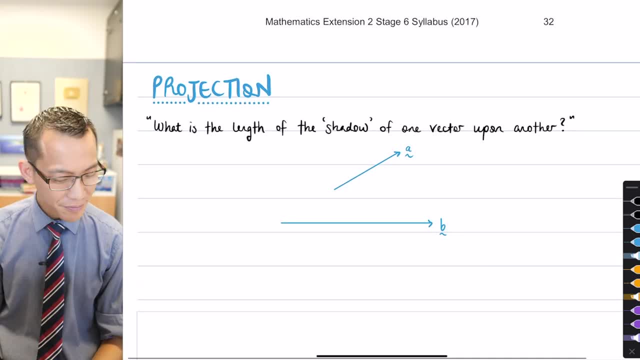 love you to do is start by drawing for me a pair of vectors. You can make them much like the vectors that I've drawn here, but part of the point of everything that we're doing with vectors is you can do it with any arbitrary vector or vectors. It's just that. 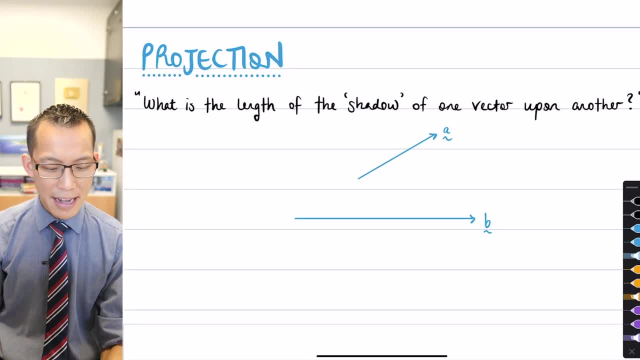 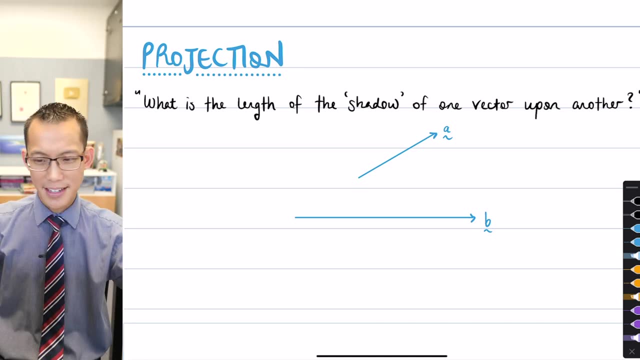 I've just placed them in two spots that are reasonably convenient to me. Now for me, the first explanation of projection, because you're like throwing all these formulas and no two notation and symbols around and you've got to know, like, what's the meaning of the thing. 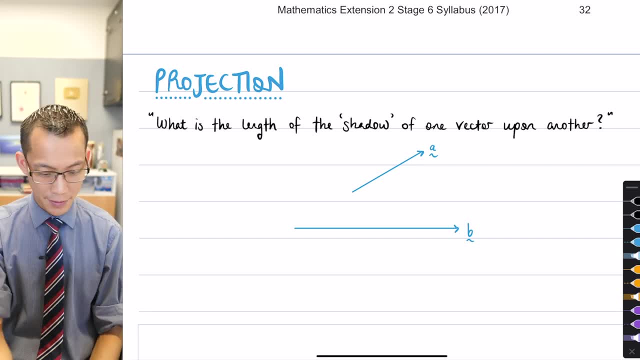 you're doing okay. The way this was explained to me the very first time is this sentence I've written here: right: When you are projecting, the first thing you do is you work out what we call the scalar projection. I should actually just jot that down for you: The scalar projection. 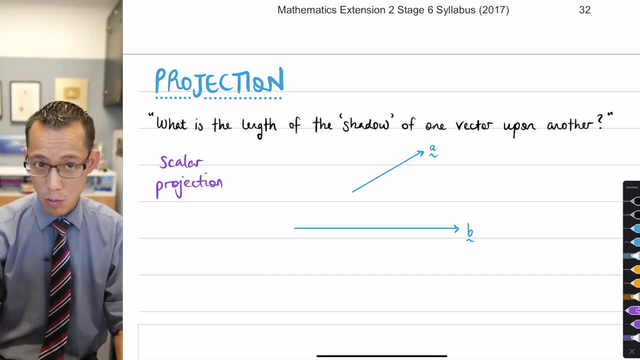 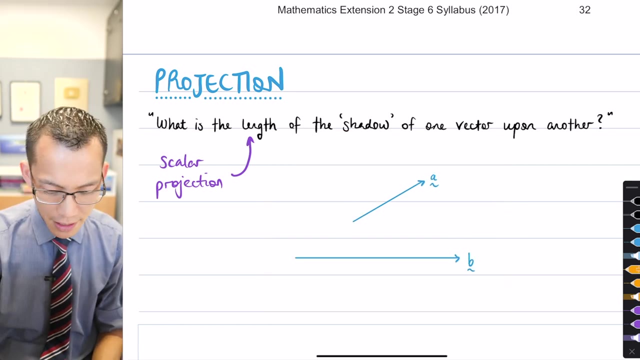 and, like all scalars, it's a one-dimensional quantity, and that one-dimensional quantity is the length of the shadow that one vector casts Just upon another, as it were. So what I want you to imagine is- maybe I'll move this down just a teeny bit, If you can imagine, you know, the sun hanging out here and it's shining. 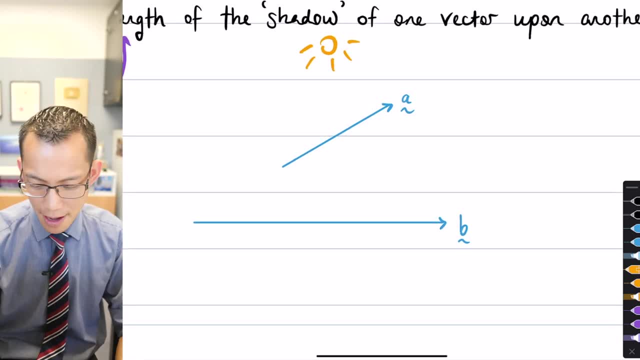 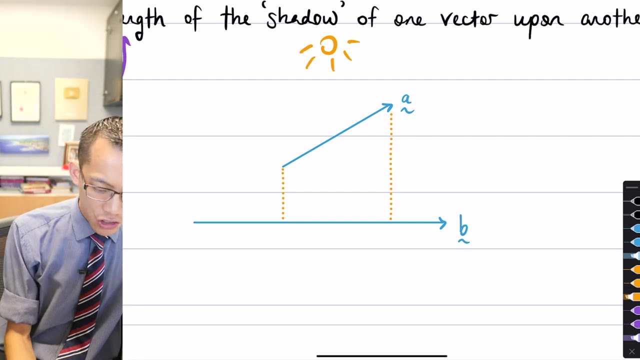 down upon these two vectors and you can sort of, in fact, let's draw this on right- You can imagine this top vector A casting a shadow onto this bottom vector B, like: so, right Now, what we're trying to work out is, hey, this shadow down. oh, that was a bit. 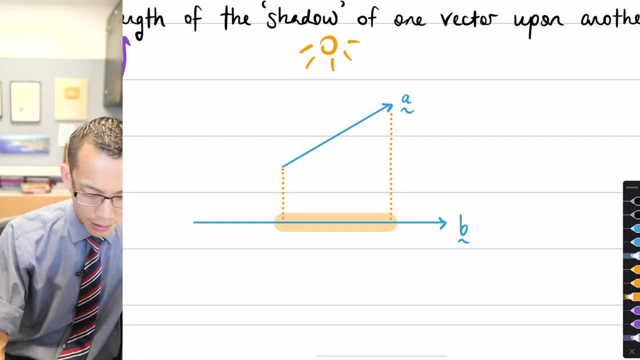 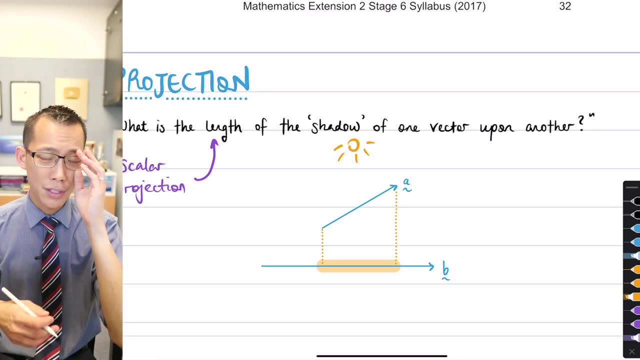 thicker than I intended. Sorry, This shadow down here. there we go. it has a length. That length is what we call the scalar projection. We're going to work that out first, and then we are going to also if we want to include the distance. That's why I just worked out. We're going to include 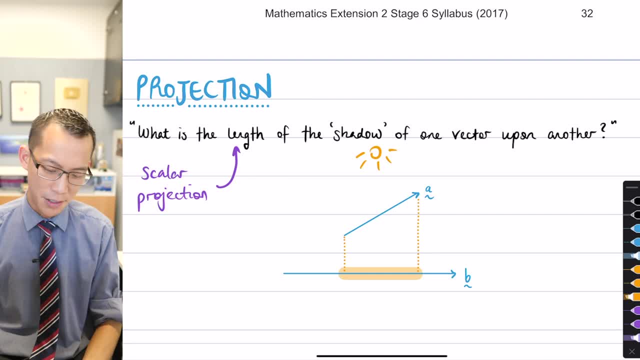 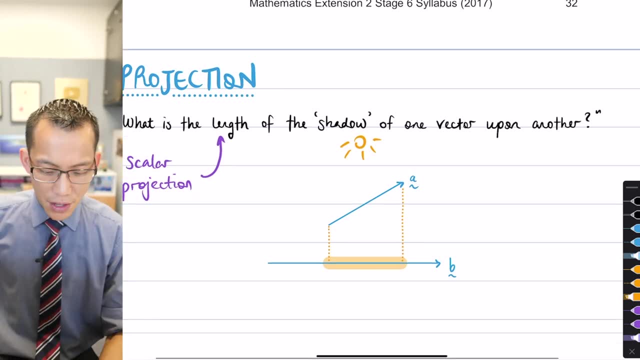 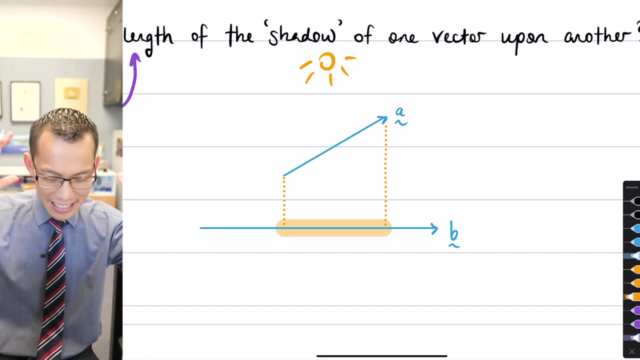 the direction of this vector in what we call the vector projection, because scalar is just a length. The vector projection is when you send it in a particular direction, right? So how does one go about doing this, If there's any, any sort of ideas kicking around from when you encountered this in 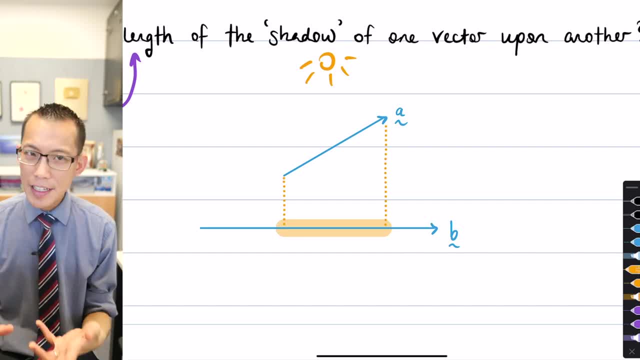 extension one. what I'm going to do is I'm going to do this from scratch and it will feel a little bit theoretical. I'm very deliberately not really going to give you a worked example on this, or maybe just a very brief one, because it's just the idea that I want us to focus. 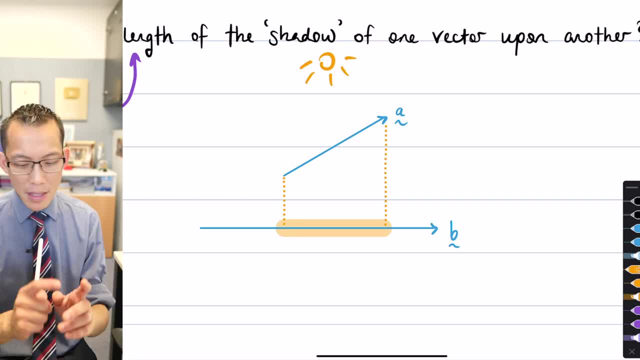 on and the geometry and the relationships between this. okay, Now, don't forget, we're in three dimensions, but even though we're in three dimensions, you can always find a plane. that Okay, Two vectors will sit in. Do you remember? I, Mrs Arles, I don't think you were in the. 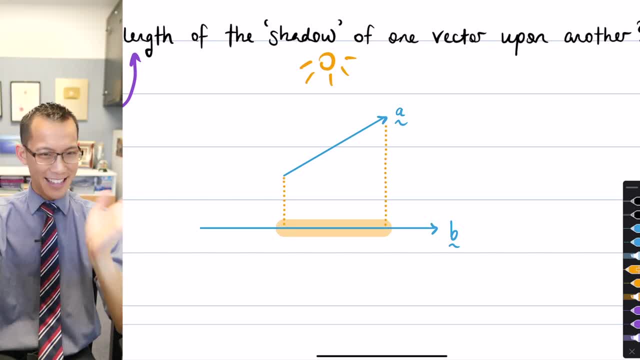 room, but I asked Ryan and Sean to arbitrarily- Yep, You saw the recording, Yep. So if it's hard, you need you need more hands, basically, which is why the two of you guys were were perfect. So for any two arbitrary vectors facing in any direction, we can find. 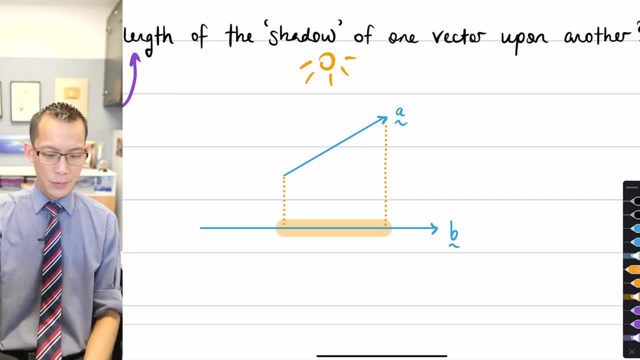 the plane that they both sit upon and that, as it were, is our piece of paper that we're looking at at the moment. Okay, So, even though I'm in three dimensions, I can still reason in two dimensions. Now, what I'm going to do is I'm going to use the dot. 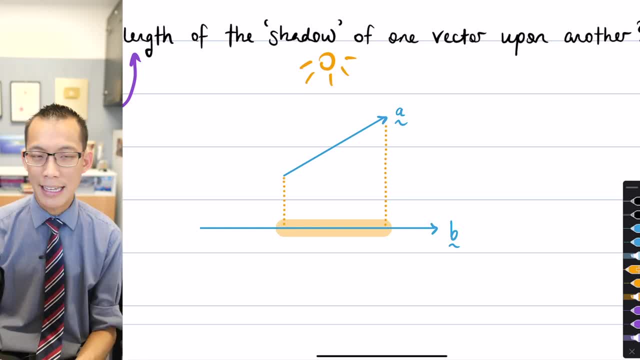 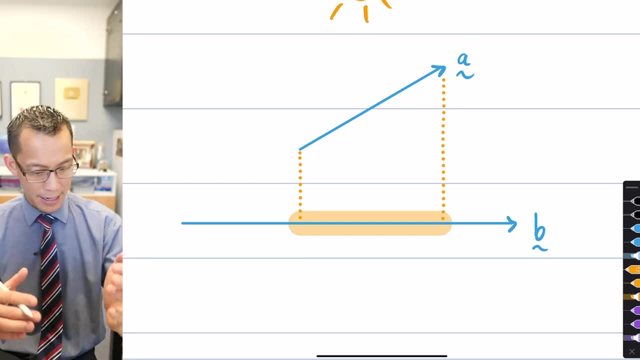 product to help me work out what the length of this shadow is, And here's how we're going to go about it. right, The dot product helps us work out, As you can see here, like there's an angle between A and B. If A was parallel to B, don't draw this, but just suppose A. 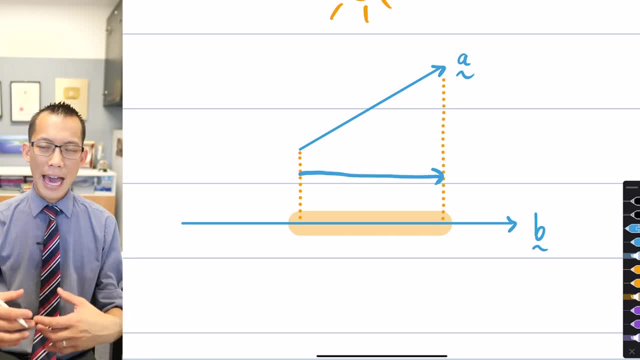 was parallel to B, like. so then that the length of that shadow. it's kind of like you don't need to do any working because the length of the shadow is just the length of A right. But of course normally we're considering when A and B aren't. 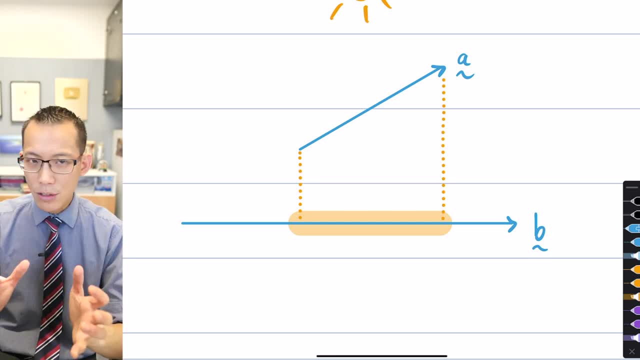 parallel. So we need to work out this relationship between the angles of those vectors, right? So what I'm going to do, and I'm going to ask you to follow here with me, is put a few constructions on here to help us. Now, what we'll do is we'll say: first we're going. 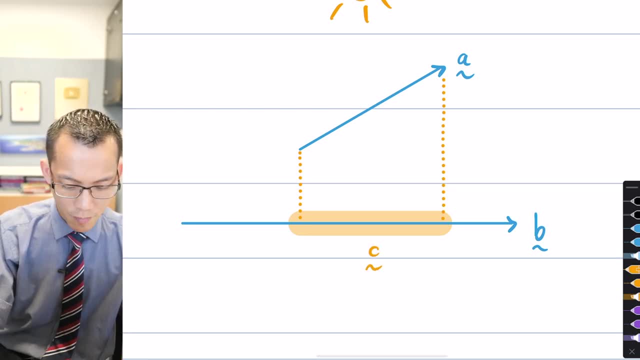 to try and work out this, this vector C. I'm going to call that the shadow right. What I'm really going to start out working out is what is the length of this vector right? That's the length of the shadow right. 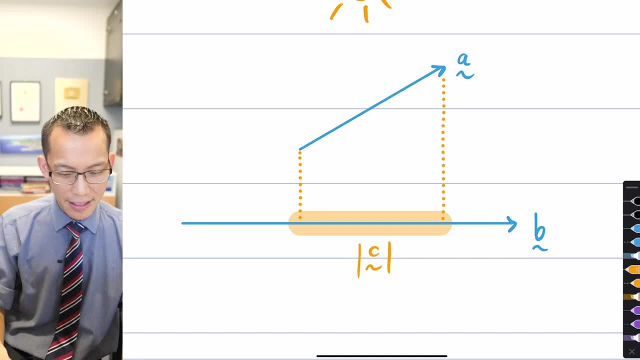 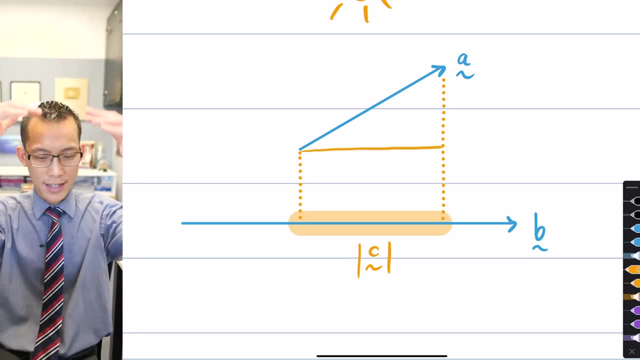 Now I can see that same length is actually. it appears in another place. If I go up here, it's sort of slide the shadow up towards the top vector right. This, this vector up here has the same length right Because it's just opposite sides of a rectangle. The reason: 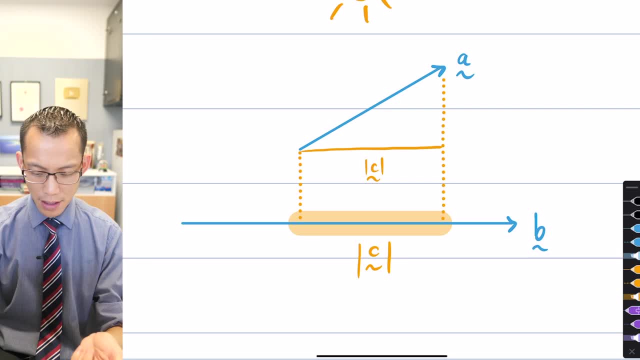 why this is helpful is because I can now match this up with the angle between this sort of repositioned vector. C is going to be the same as the angle between A and B, And if you can imagine picking up A and putting it tail to tail with B, you'd get the same. 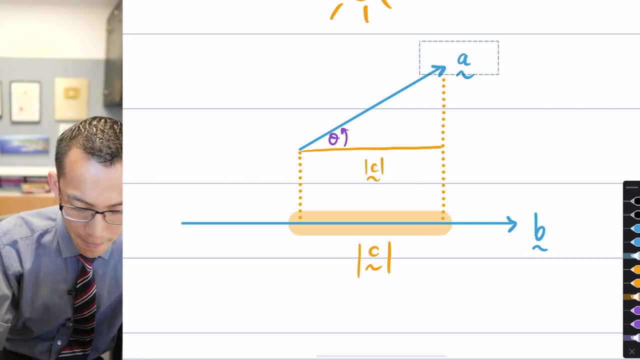 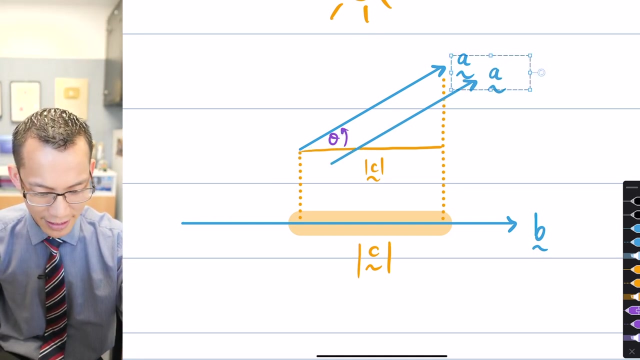 theta right Like it's going to be. I guess I can. you don't have to draw this, but if I duplicated this over here, you can actually see. it's that same theta right, It's just in a different spot. Okay, So let me get rid of that, because that's unnecessarily clouding. 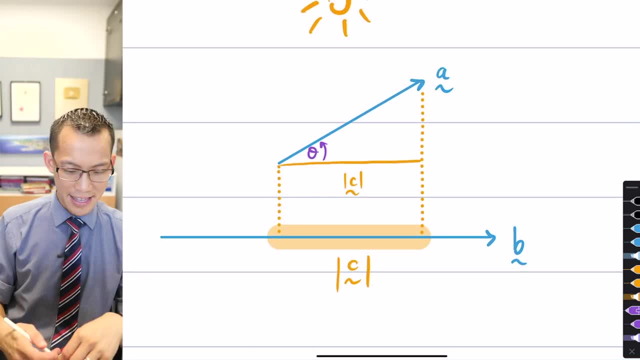 our diagram. There we go. So how do we work this thing out? Well, I've got the length. I can work out the length of this vector Using just the magnitude of any vector, And you can see here what I've got actually is. 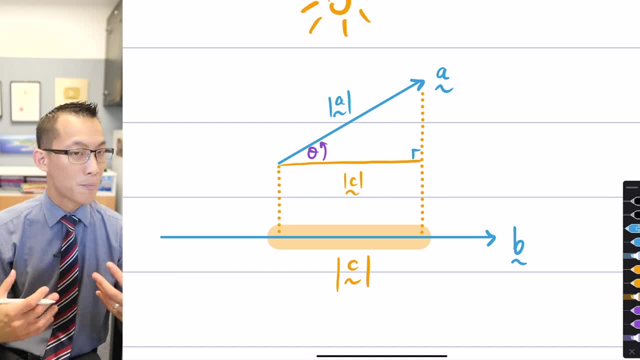 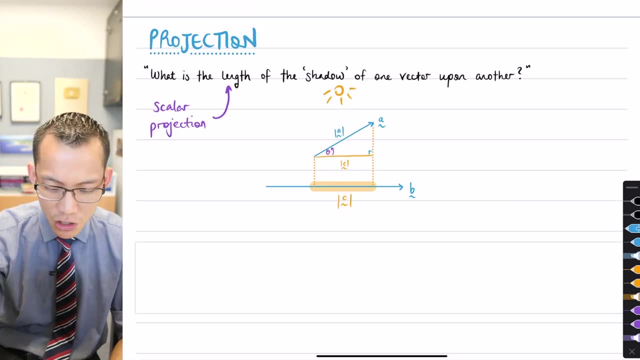 a right angle triangle in here, So I can use some pretty simple trigonometry and relate this to the dot product, right? So let's actually jot some of this down. I'm just going to use my space on the right hand side because I've not left myself enough space, So I'm just 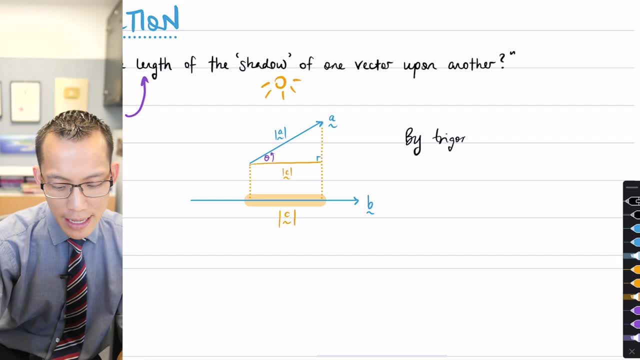 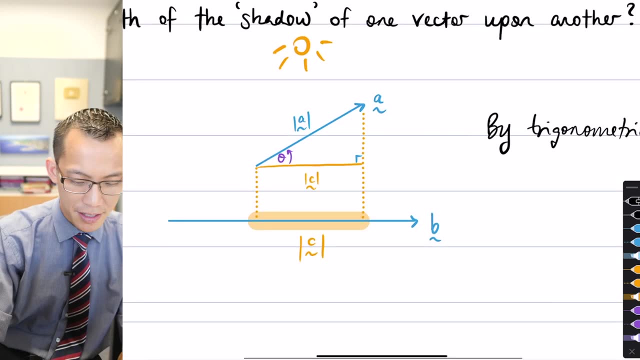 going to say by trigonometric ratios. what is the particular ratio that connects the two sides that I've got Two sides, that I've got here and I fixed my laser pointer so it should work. I've got A and I've got C. What's the ratio? 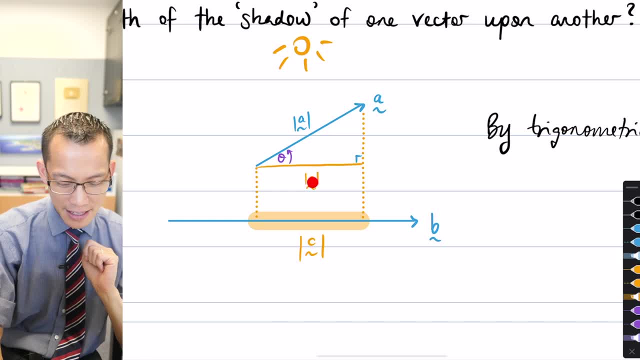 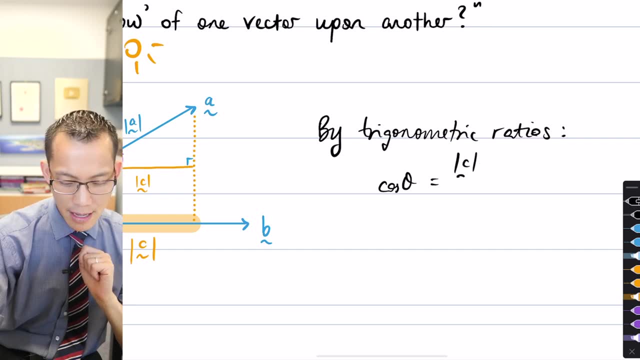 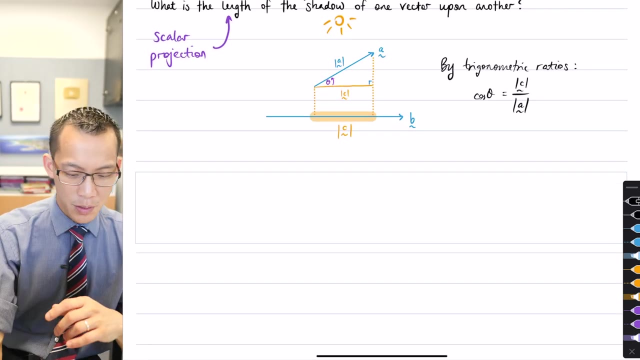 Cosine. Yeah, fantastic, The cosine is adjacent over hypotenuse. So I'm just going to say: cos of theta is equal to C, that magnitude on A like. so Now this is really helpful because what I can basically say is: hey, that cosine of theta that appears in the dot product. 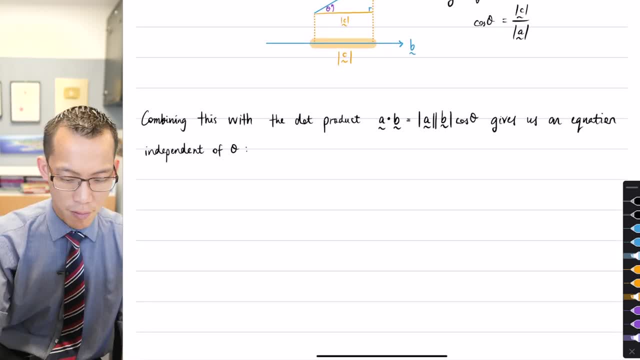 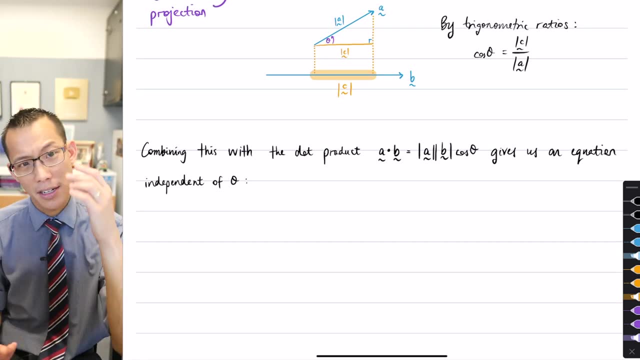 right. So I can say: let's use the formula for the dot product that has cosine in it, so the angle between the two, and that'll give me an equation that doesn't have thetas in it, And that's really nice because we tend to get our vectors in component form right. So if I've got all, 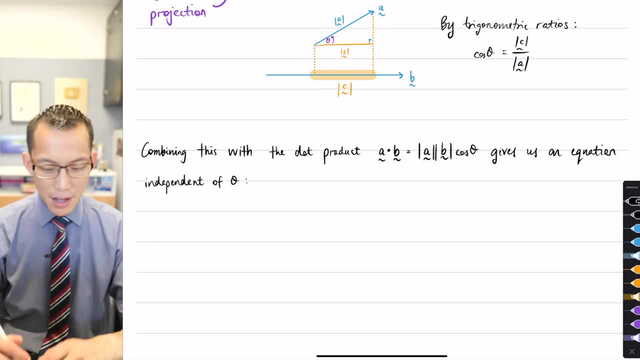 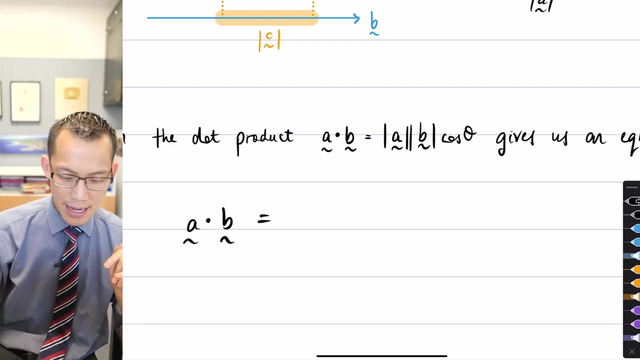 the components, then I don't need to work out theta separately. So here's what I'm going to write. I'm going to say A dot, B. What's that going to be equal to? Well, I would normally say magnitude of A, magnitude of B, and then cos theta, But I don't need to say cos theta. 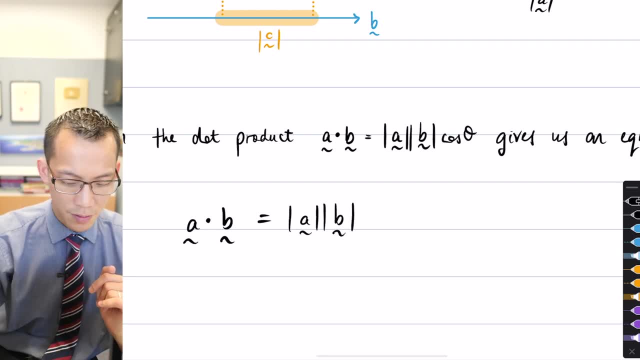 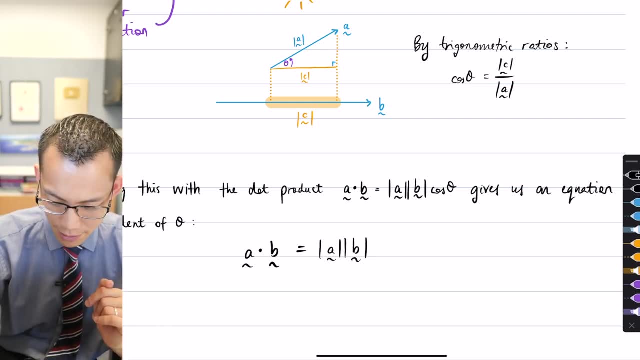 because I've got an expression for that Magnitude of A, magnitude of B. I've got an expression for cos theta up the top here. Oops, Let's highlight properly, shall we Can't reach it? There we go. I've got this. 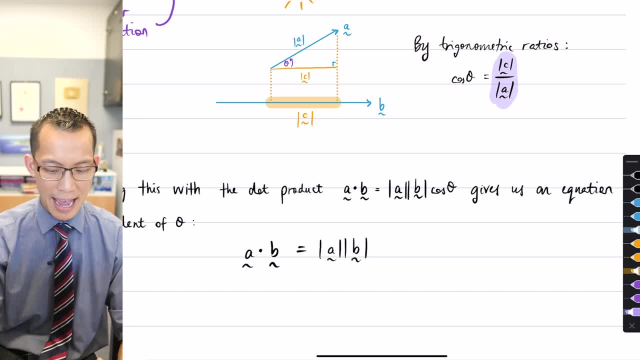 expression up here which is the same as cos theta. It's equivalent, but it just doesn't have any of the angle in it. So let me just grab that Again. sorry, I'm just going to be a little bit cheap and do that. 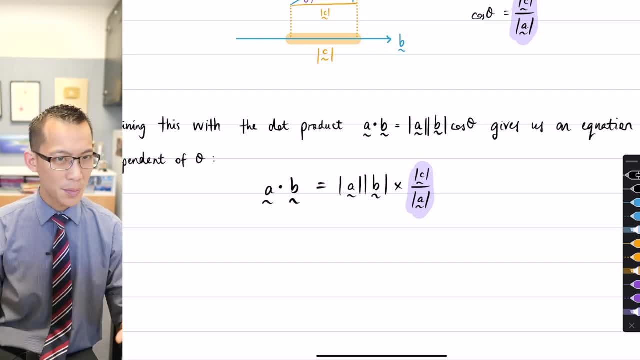 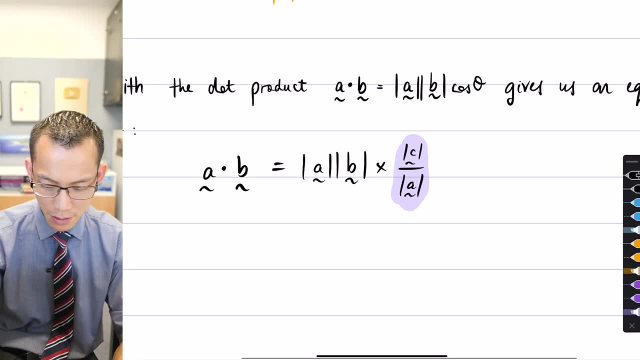 And hopefully you can see. you're like, oh, I can do some cancelling here, right? So what I'm going to do is on the denominator there you can see that magnitude of A it's going to cancel with the magnitude of A that comes from the dot product formula. So now what? 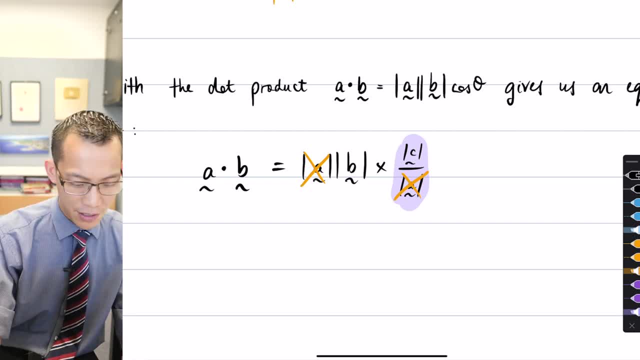 I've got here is just, and I'll write this on the left-hand side, because if you remember the thing I'm trying to work out, the length of the shadow, it's this magnitude of C. So I'm going to get towards making that the subject, So I'm going to write that on the left-hand. 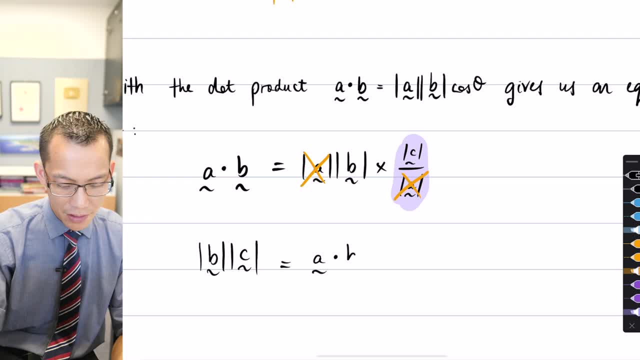 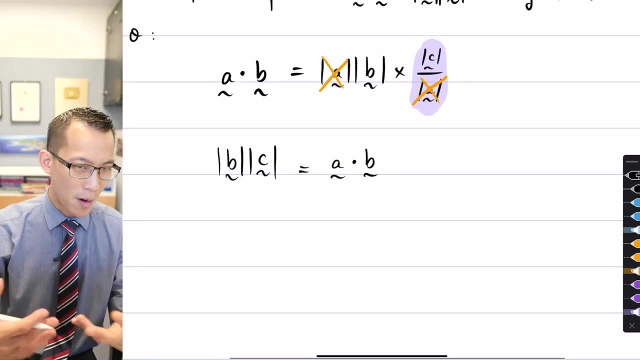 side That's just equal to A dot B, because all the rest of the things have cancelled. Okay, All right, Now let's keep going. I'm now going to say: if what I want is just the magnitude of that vector, the length of the shadow, I just have to divide through both sides by 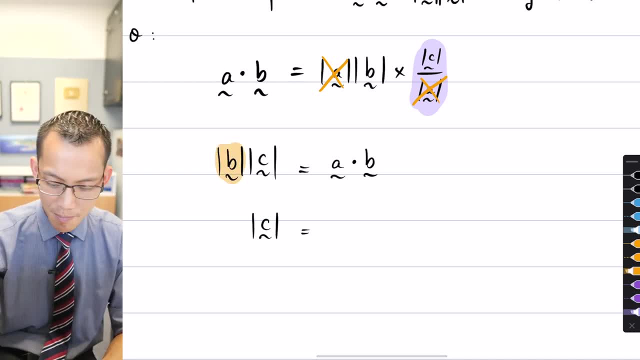 the magnitude of B, which I have over here, right? So let's go ahead and write that. So I've got A dot B on the numerator and then I'm dividing by the magnitude of B. Okay, This is fine, This is all true, But I can write this in a slightly simpler form, if you. 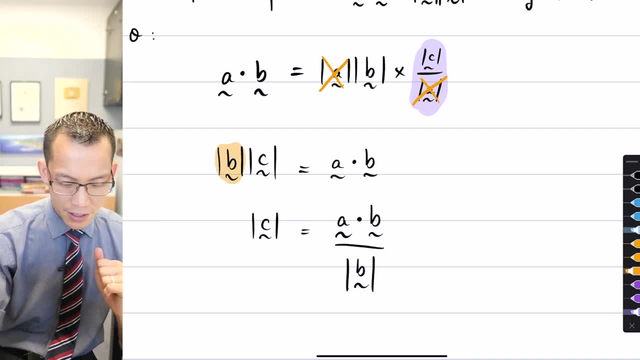 can help me remember that. actually, if you take some arbitrary vector and you divide that vector by its magnitude, what do you get when you do that process? If you divide a magnitude- sorry, a vector- by its own length, Yeah, very good, This gives you the unit vector. 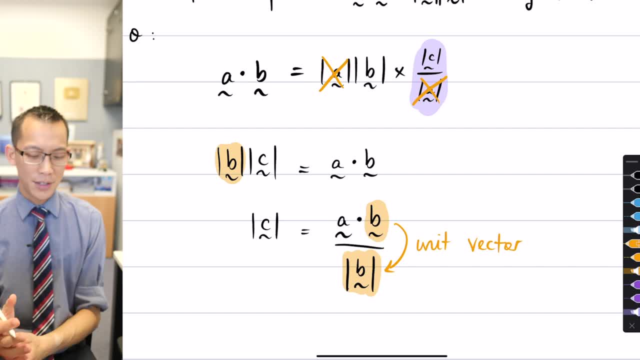 or I should say the corresponding unit vector for that. Because if it was a vector off at this particular angle and it was 15 units long, and then you divide by 15, well, now you've got, the direction is still there. You haven't changed the direction at all, but you've divided. 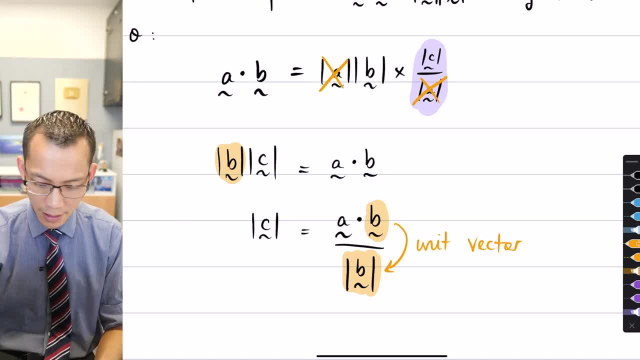 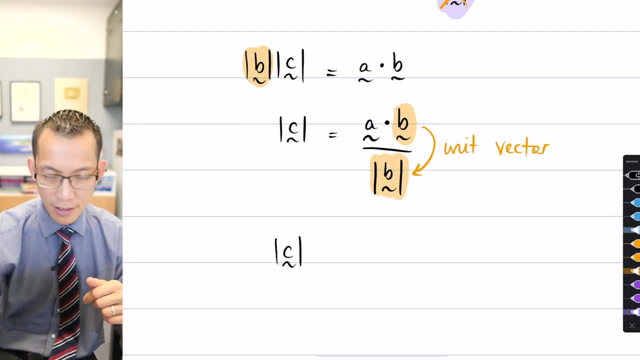 by 15, so now it's one unit. So that's what makes it the unit vector. Okay, So what I can do is I can say: all right, this scalar projection, the length of the shadow, the magnitude of C, they're all the same thing. What that's equal to is A dot, and if you remember, 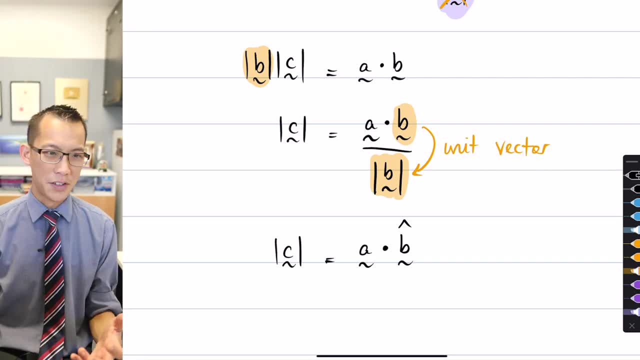 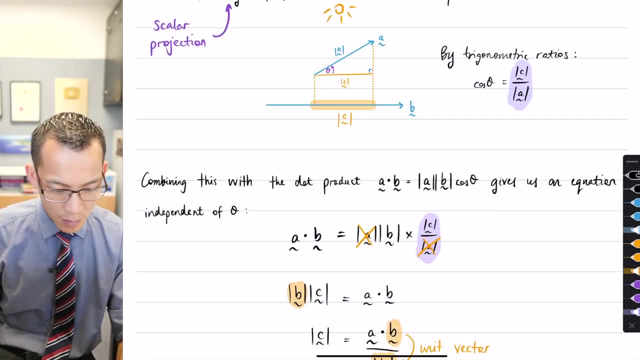 we write the unit vector as the same as B. Okay, With a hat over the top, Okay, So there's. there's the unit vector there. So this thing here is what we were describing before. Where did I write it? Yes, I wrote it in purple. 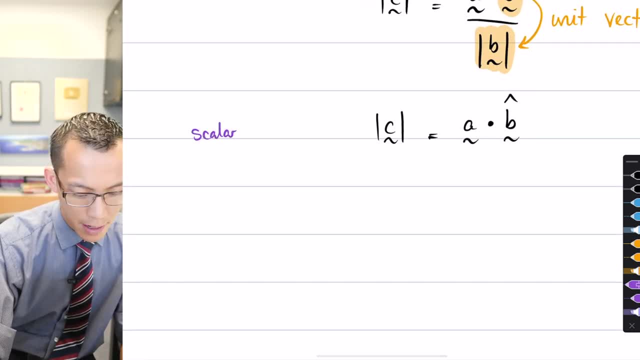 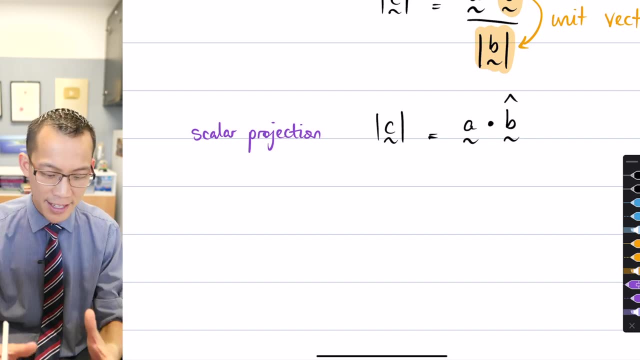 This thing is what we call the scalar projection. Remember, when you do this dot product, all you get is a number at the end right, And this particular number, this scalar number, is the length of that shadow. Okay, So what I can do is I can just sort of extend that just a little bit. And if I said just 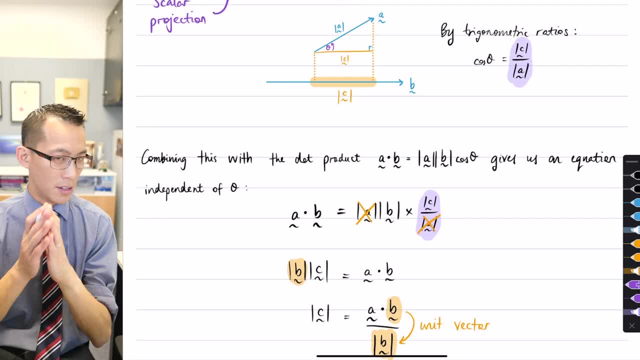 going back to our original diagram, if I wanted to know not just the length of the shadow but like where is that shadow facing, then all I have to do is multiply by the direction part. right Now, if you have a look here, the direction is given by B, but I don't want. 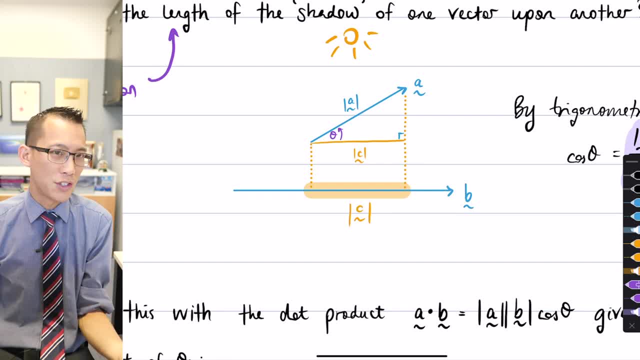 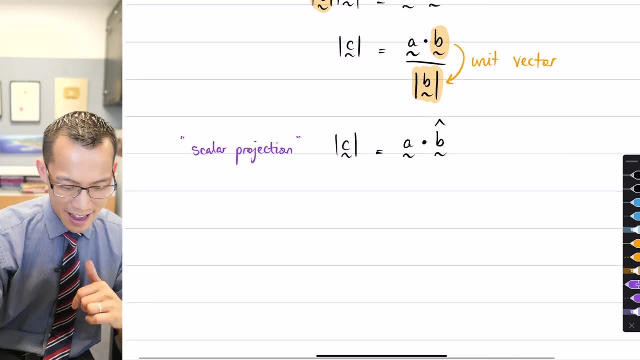 to have like the length of it, because that would change the length of the shadow that I've just calculated. So what do I multiply by to get the direction of B without any kind of change in its magnitude, Just the length of the shadow? It's the unit vector again, right Now. this is important because what we're working